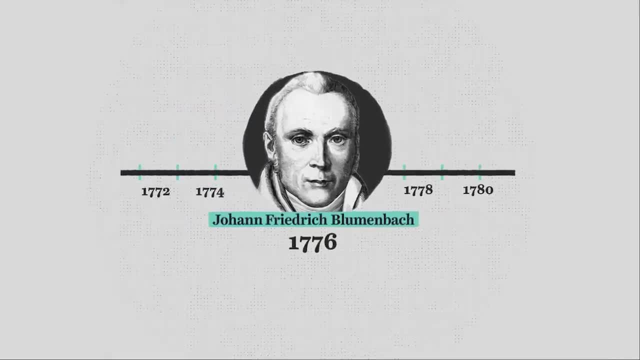 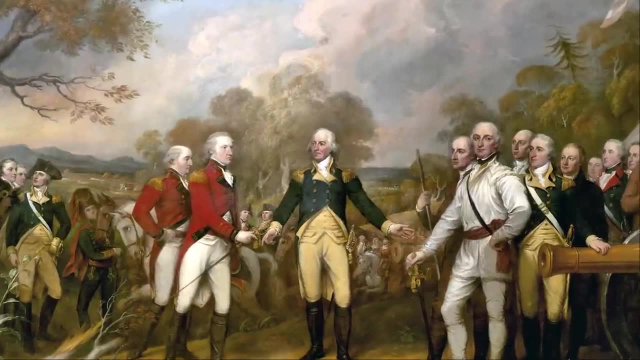 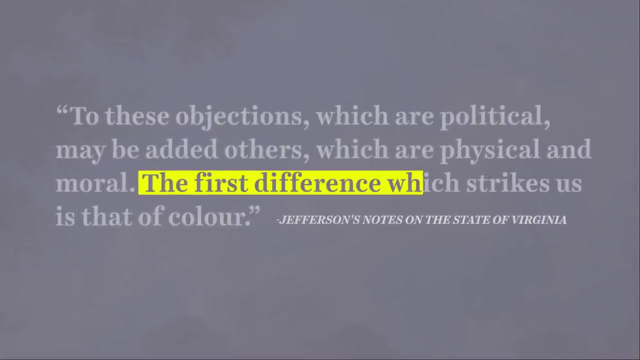 to race was a German scientist around 1776.. He came up with five different groups according to physical appearance and geographic origin of their ancestors. Americans of European descent eagerly bought into this type of thinking. around the same time, Some historians have said the idea that there were different races helped them resolve the contradiction. 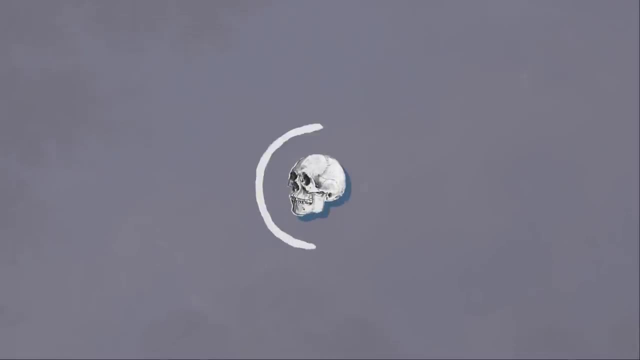 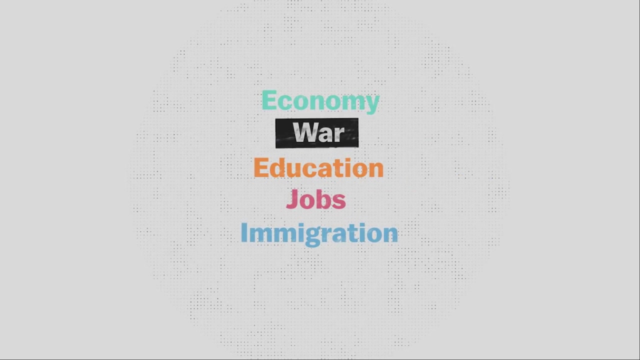 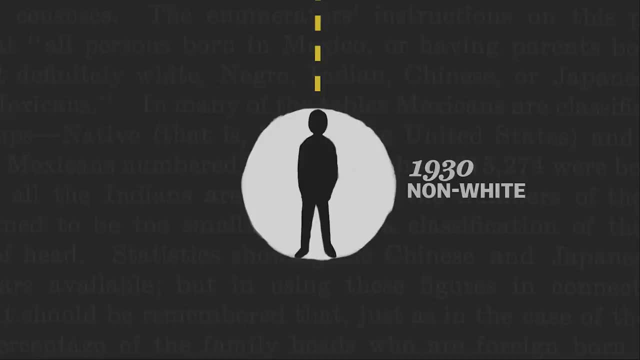 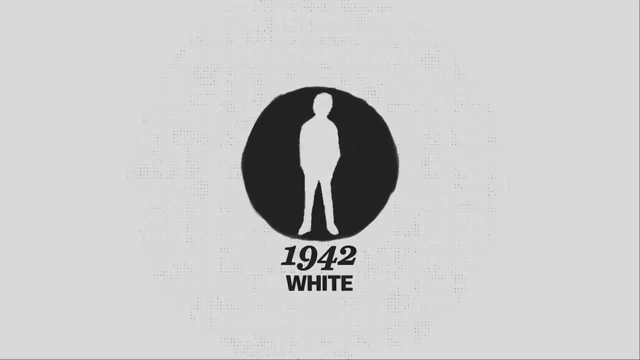 In the United States in 1929, you were considered white. Then the 1930 census changed that to non-white to limit immigration. Later, when the US needed to increase its labor force during World War II, these people were switched back to white. And what it took to? 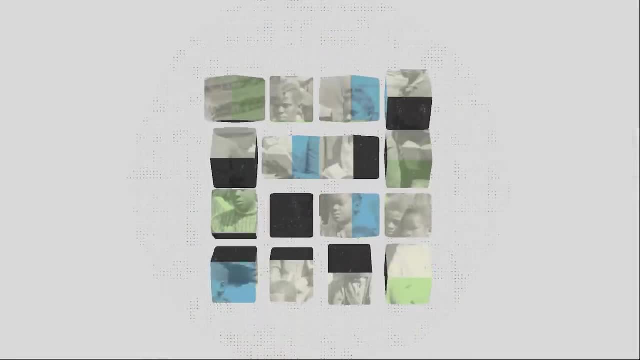 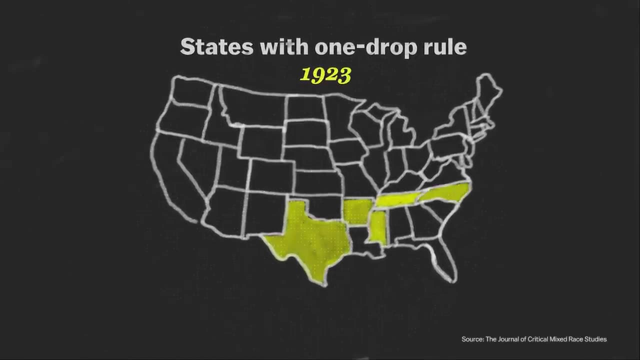 be black once varied so wildly throughout the country, from one-quarter to one-sixteenth, to the infamous one-drop of African ancestry, that people could actually change races just by crossing state lines. Then suddenly, in 2000,, the government decided that a 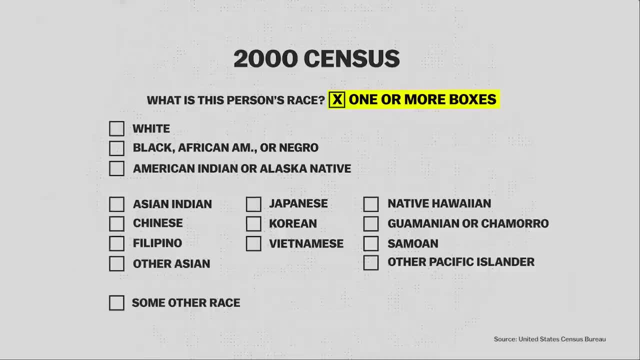 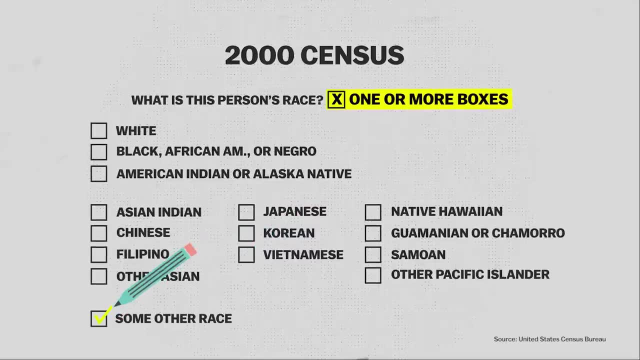 Americans could be more than one race and added a multiracial category to the census. This has left many Americans scratching their heads when it comes to selecting who they are. As many as 6.2% of census respondents selected some other race in a 2010 survey. 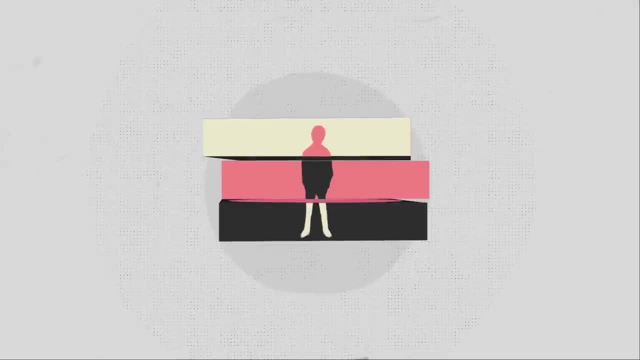 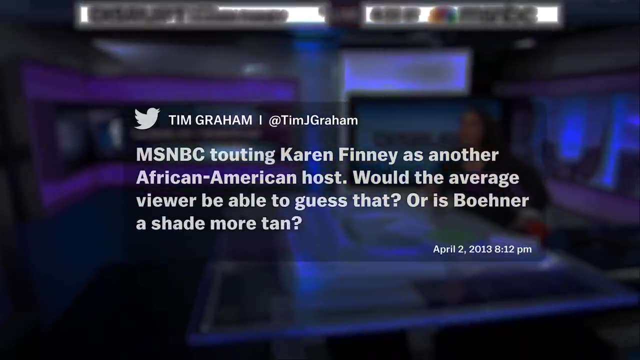 The idea that someone might look one way and identify another way, or that they might be really hard to place in a racial category, is not new. This is why there was a public debate about whether MSNBC's Karen Finney could say she was black, or how we can't even agree on the racial label assigned to the President. 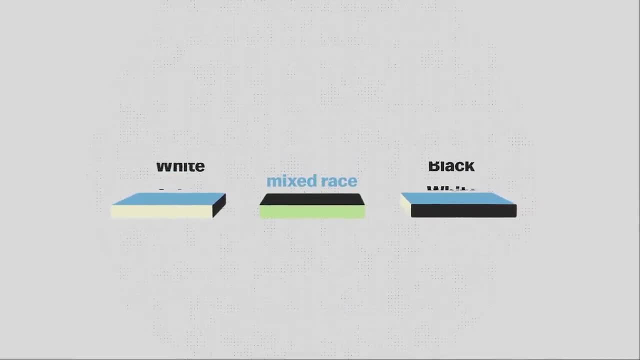 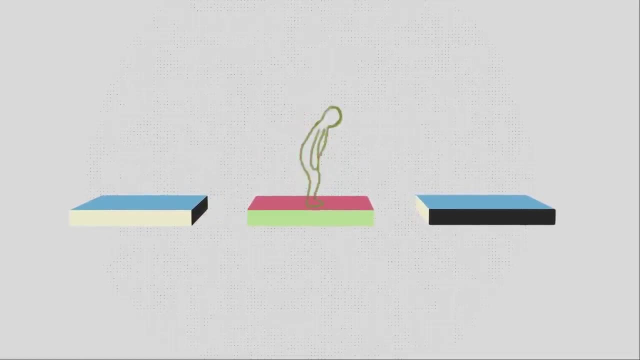 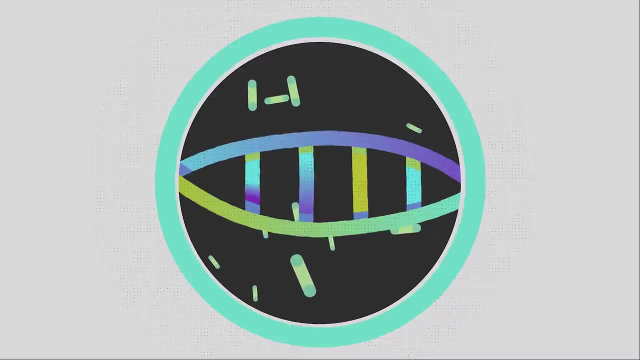 of the United States. Of course, many people feel their racial identity is very clear and very permanent, but the fact that some people have changed theirs and that no one can really argue with them shows how shaky the very idea of race is. This is all because there isn't a race chromosome in our DNA that people can point to.